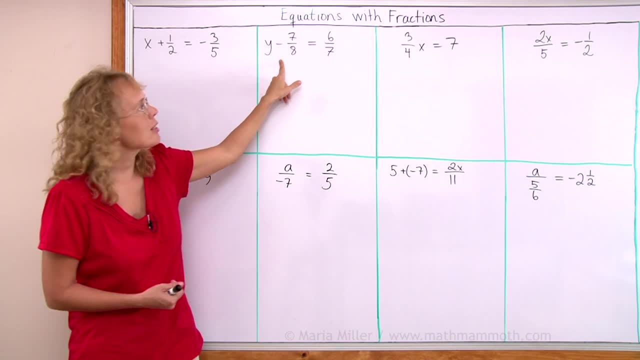 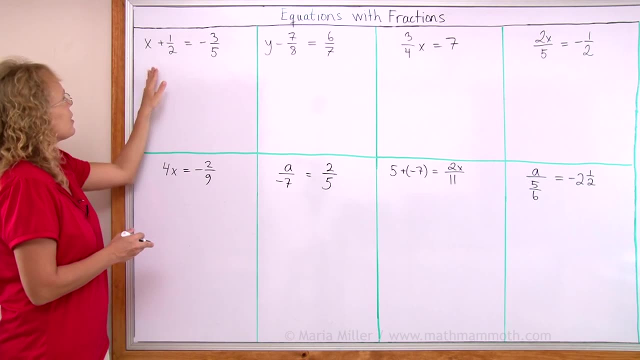 is called a subtraction equation, because from the variable we subtract something, and over here we have a multiplication equation and a division equation, simple equations. And since half is added to the variable, we need to subtract half from both sides to solve this. So I will subtract one half, subtract one half from both sides, and then we get. 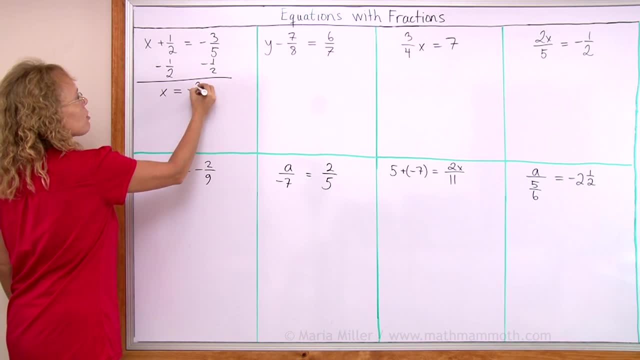 x alone here, which is what we want. Over here we have minus three fifths minus one half to calculate. no, So this is a fraction subtraction and the denominator is different. So I need to find a common denominator which is ten will work, okay. 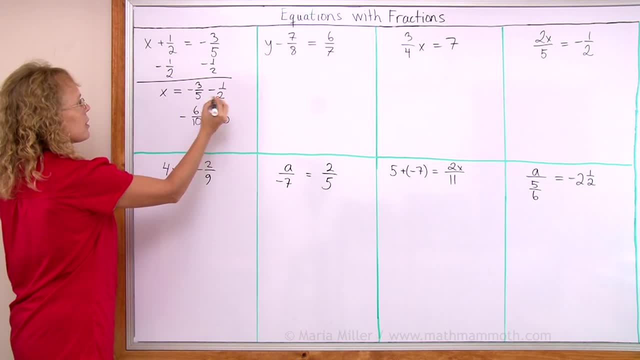 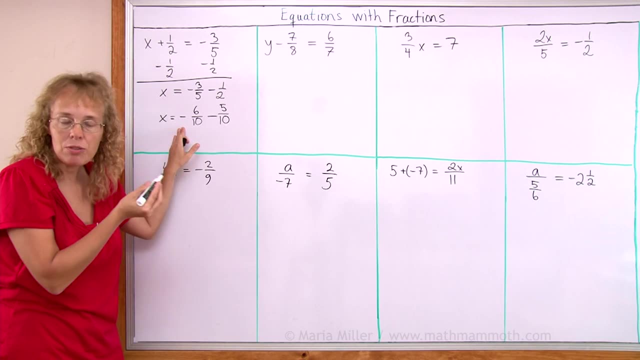 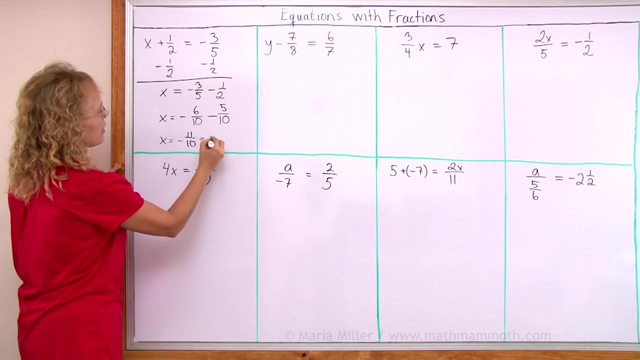 And I will get six tenths minus five tenths. So we get minus six minus five. it is minus eleven or negative eleven tenths, Or you can write it as a mixed number: negative one and one tenth And you should always check your answer. 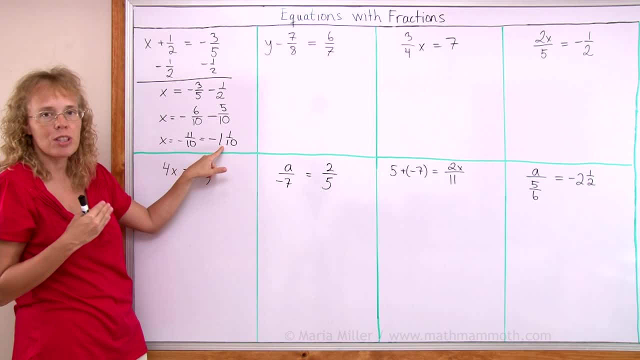 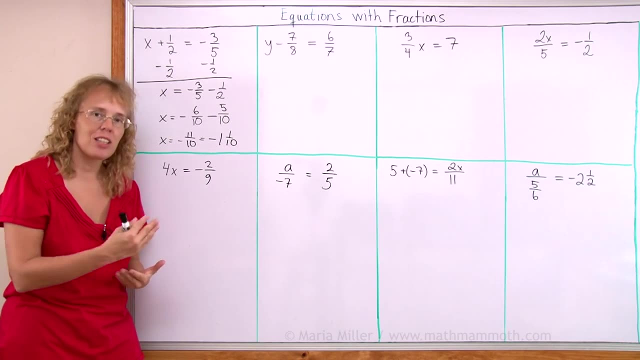 Check this rule. check if this really is the solution for your equation by substituting it over here. I'm not going to take time to do that calculation now because of the sake of the video, so it doesn't get too long, But that is what you should do every time. 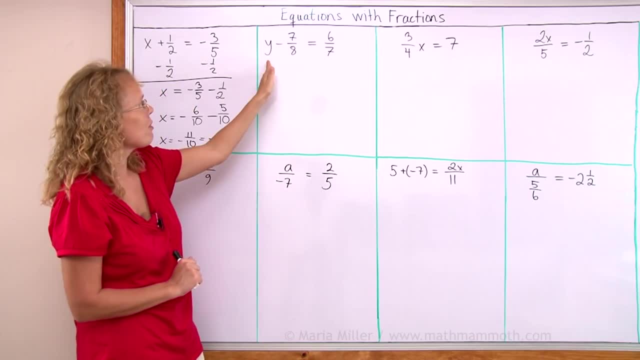 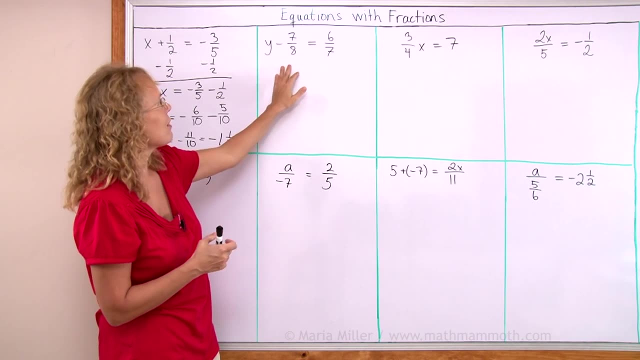 when you get your solution. Here we have a subtraction equation from the variable seven eighths is subtracted. So to solve the equation we will add that amount to both sides. We will add seven eighths to both sides, So we will get on this side seven eighths plus. 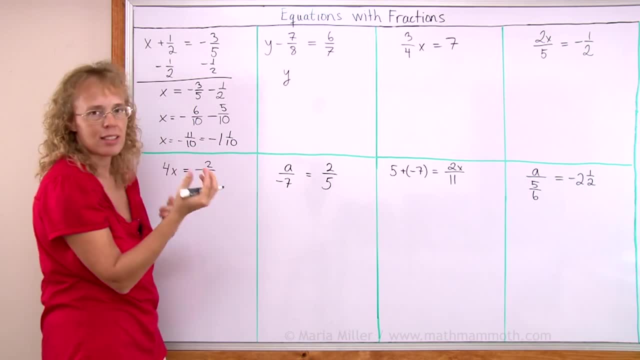 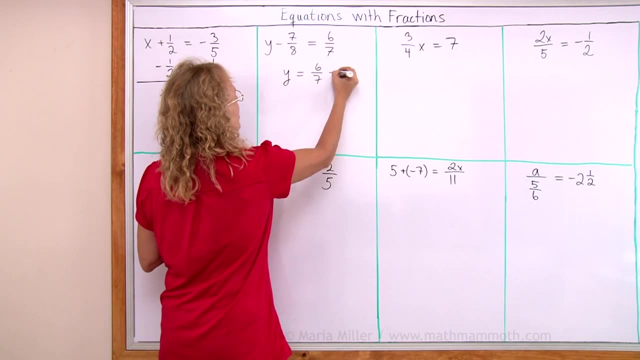 seven eighths. We will also add to both sides y along, because when we added the seven eighths, then the negative seven eighths and plus seven eighths they cancel, And then on this side we will get this plus seven eighths right. Again, a simple fraction addition that you. 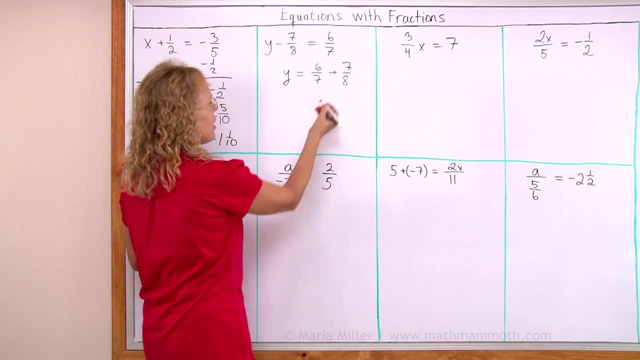 have learned to solve in fifth and sixth grades, Seven and eighth. I will need a common denominator which fifty-six will work Seven times eight. so six times eight goes here, And then seven goes here, And now 48 plus 49 is going to be 97.. 97 over 56, which, of course, as a 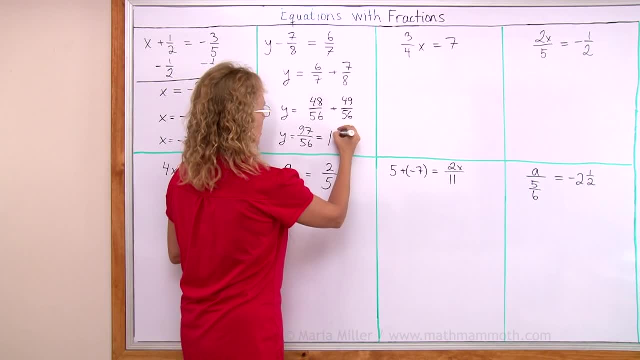 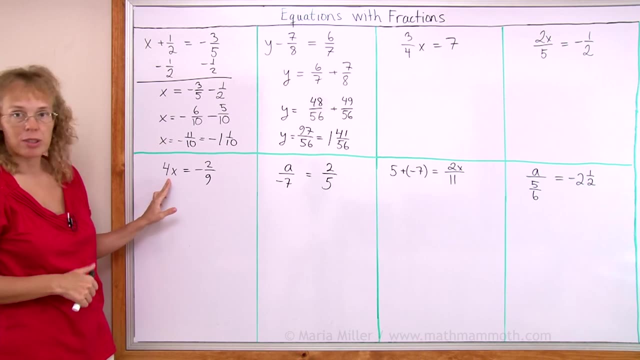 mixed number would be 1, and then 41 over 56.. This here is a multiplication equation. There's 4 times the variable. so to solve it we will divide both sides by 4, right, We will write: 4x over 4 equals now this negative fraction over 4.. This 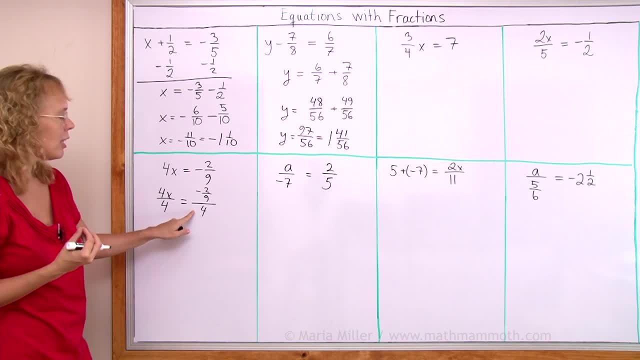 looks maybe strange if you haven't seen it before. It's a complex fraction, but all it means is this fraction divided by 4.. So that's what we need to do, Of course, here the 4s cancel. so we have x now isolated alone, And here I will write it. 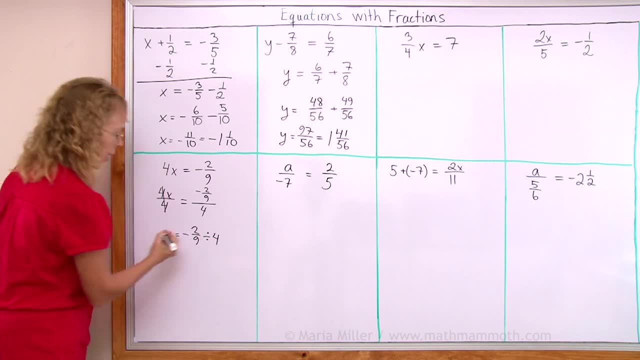 using the other division symbol like that. okay, Look more familiar now. Okay, And now we need to use the normal way of dividing fractions, which is that you change it into a multiplication. You have negative 2 ninths times and then the reciprocal of 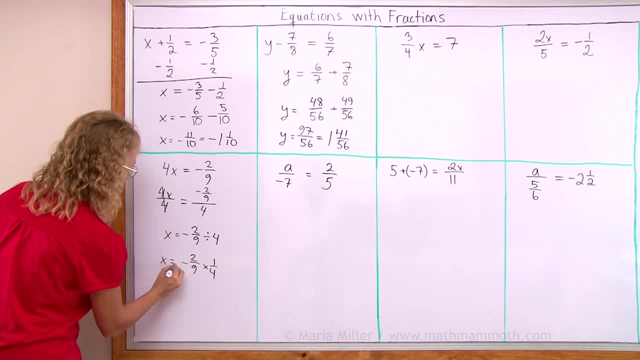 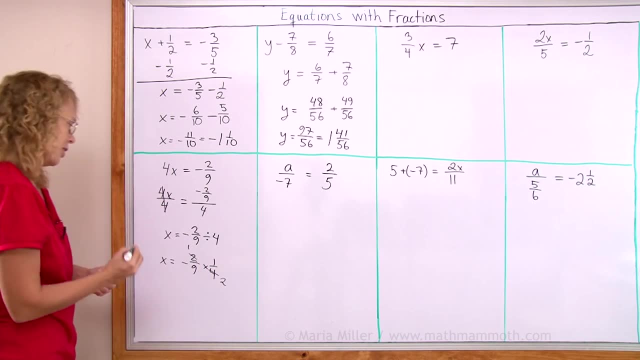 4, which is 1 fourth. So that's what we need to calculate here, And 2 and 4. I can simplify here, leaving 1 here and 2 here. So then it is 1 over 18, but it is. 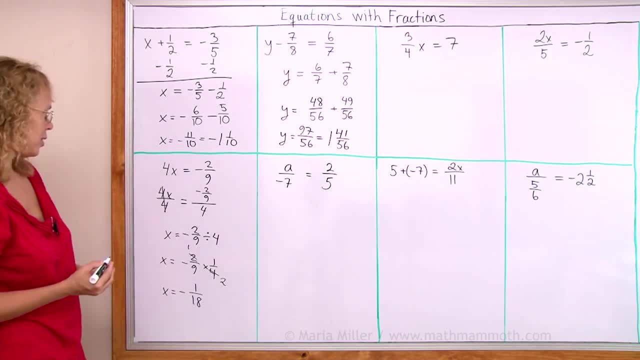 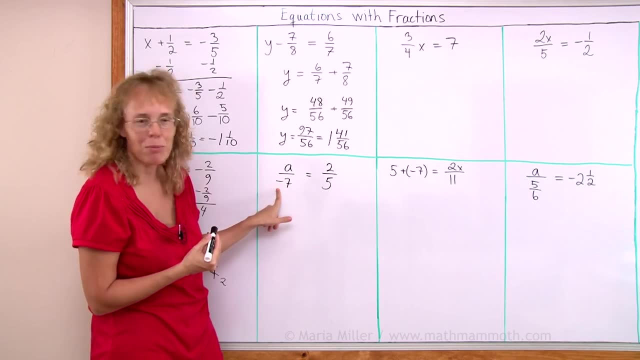 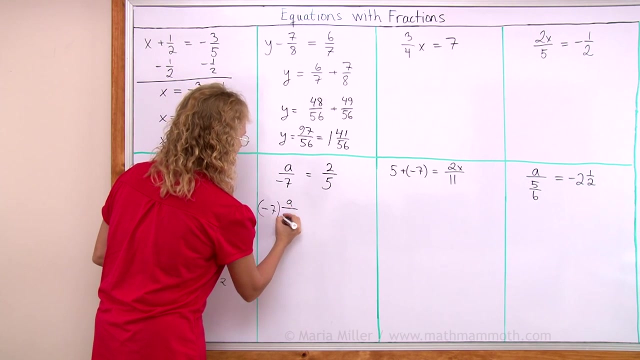 negative. Negative 1 over 18 is the final answer, And the variable is divided by something. So then we solve the equation by multiplying both sides by negative 7.. Okay, So we get negative 7 times a over negative 7. And then 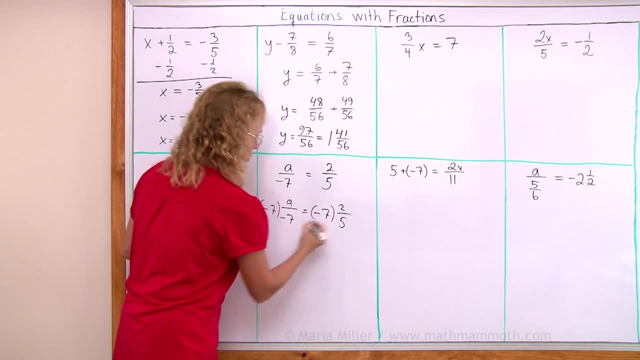 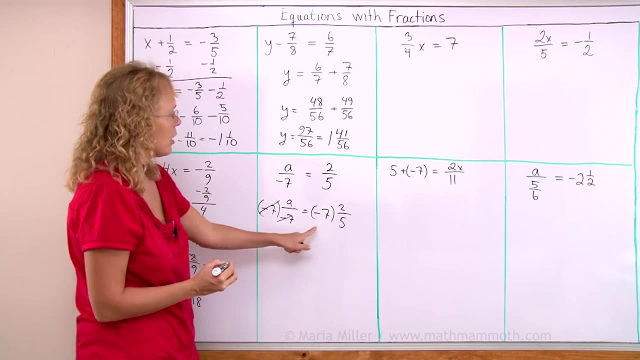 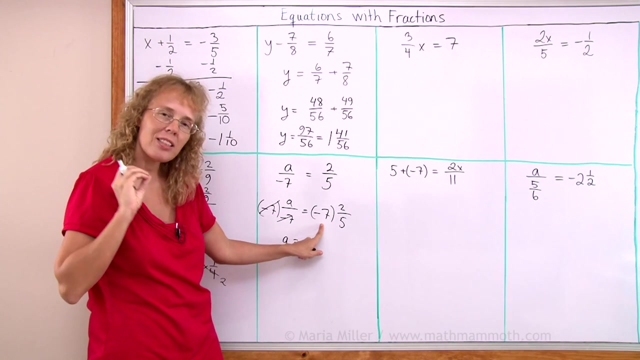 on this side: negative 7 times 2. fifths Here. the negative 7 is now cancelled, so a is now left alone on this side, which is good. Now here's a number, a whole number times a fraction, fraction. It's a negative number, so my answer will be negative, but I can calculate it as: 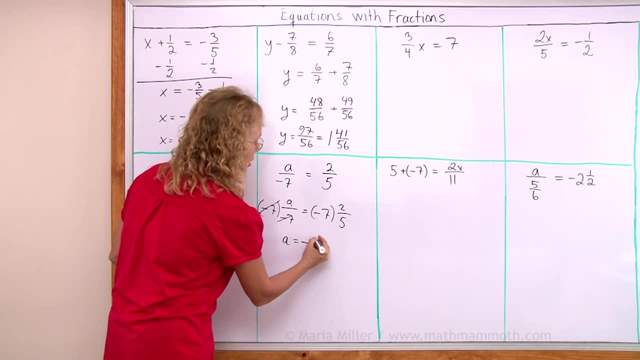 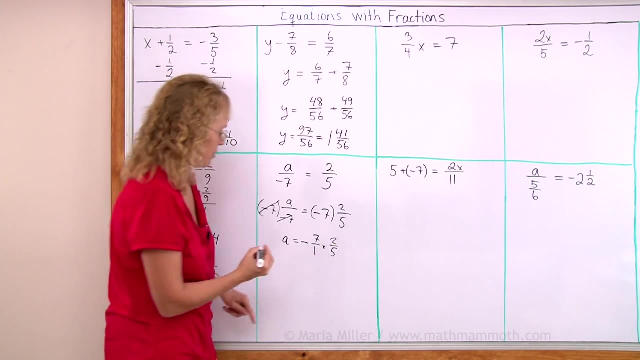 okay, it's going to be a negative answer. and then 7 times. think of it as 7 over 1 times 2. fifths, if that is easier, and we get 14 over 5. A equals negative 14 over 5, which is the same as negative. 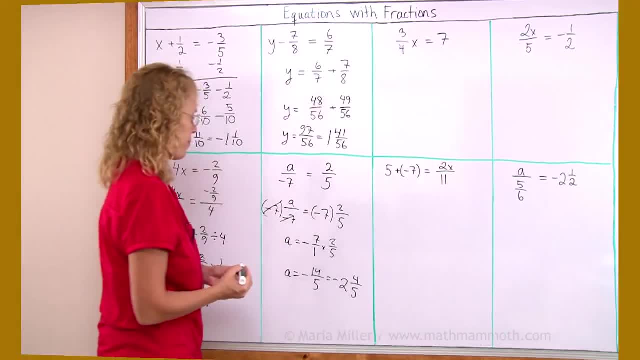 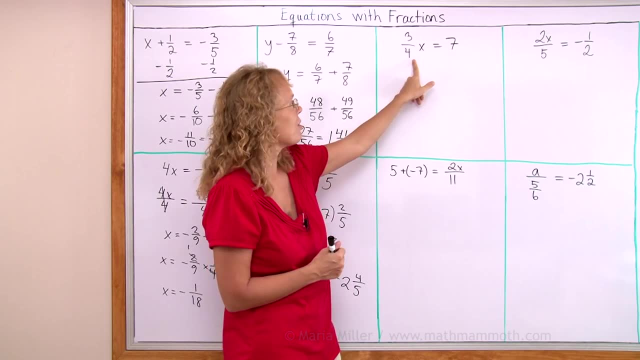 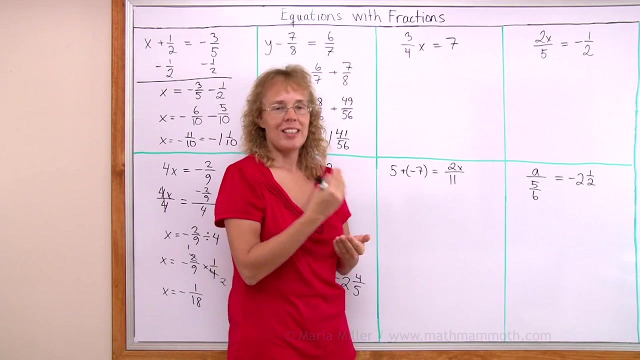 2 and 4, fifths There. This one here is a little bit different from the ones before, because now the variable is multiplied by a fraction And of course it is a multiplication equation again, so we can solve it by dividing both sides by this fraction. However, remember that when you divide, 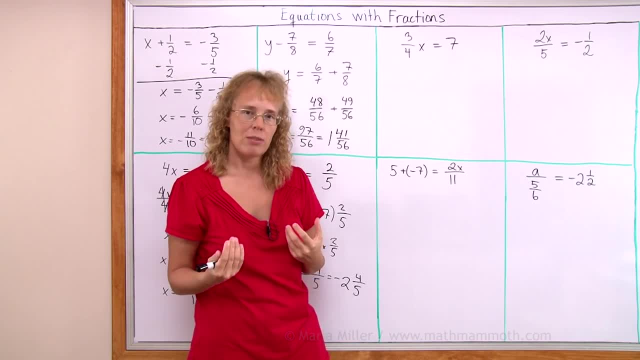 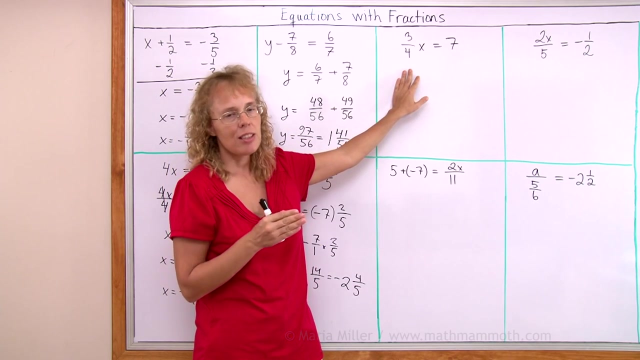 by a fraction, you always have to change that into a multiplication right. If you divide something by 3 fourths, you have to actually change the problem into a multiplication by the reciprocal right. You have to multiply by 4 thirds. So that is why in this equation, instead of dividing both sides, I will 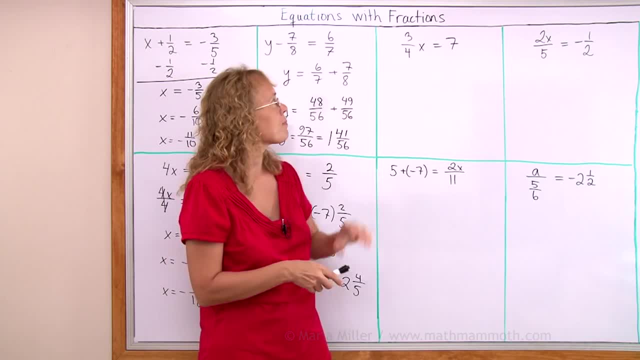 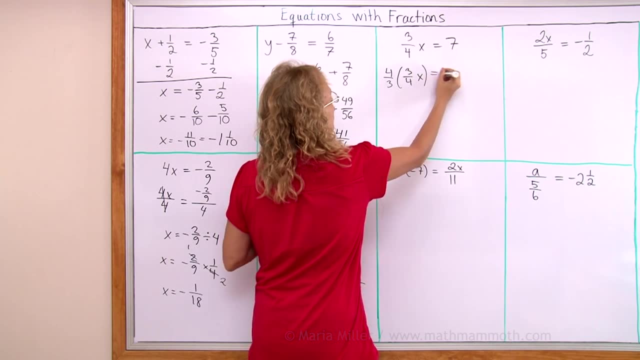 just go straight to multiplying by 4 thirds. So we have 4 thirds times 3, fourths times x, and then 4 thirds times 7 on this side, And now you can see over here there's 4,, 3,, 3,. 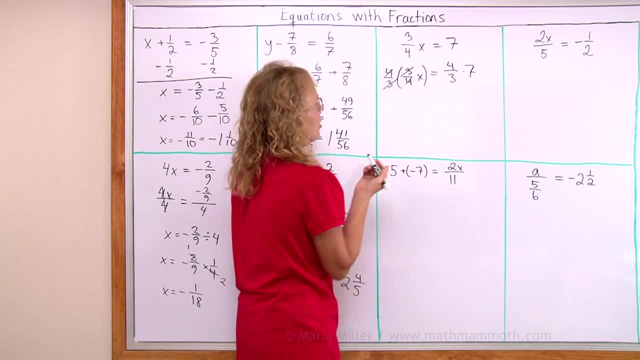 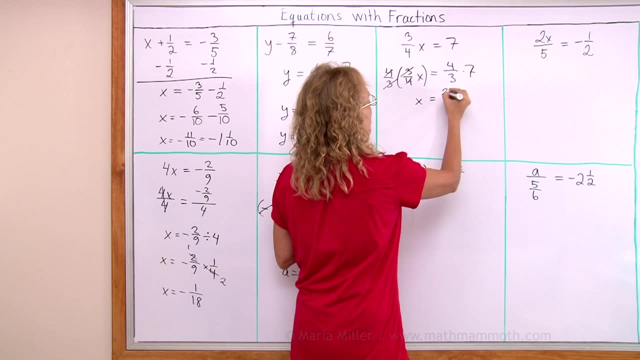 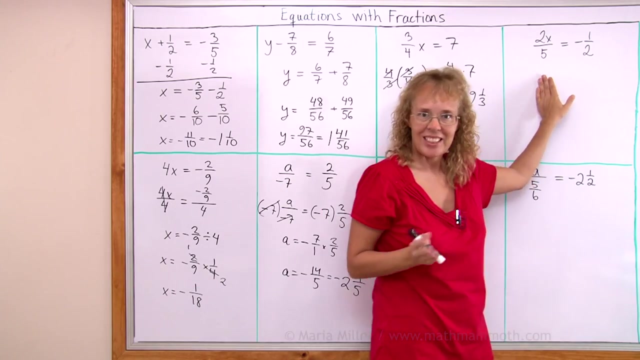 4, 4, and then we can find 4.. Before we can find the other 3, so we need to multiply both sides. So this is the same exact equation here that we did with the other three. So if you look at this equation, you can see that. 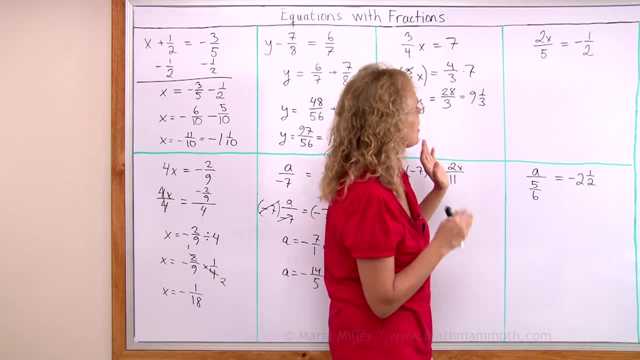 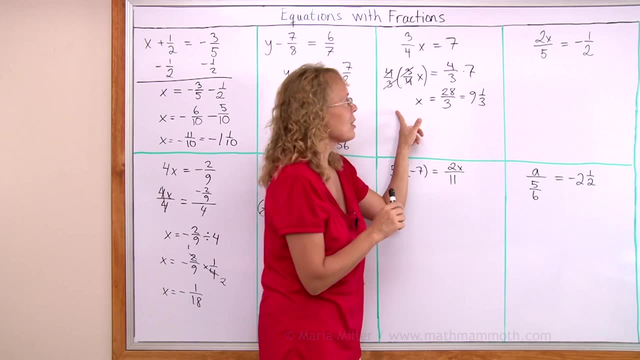 you can multiply all these things, You can see that x is going to be the same as it used to be before, the same exact equation as 2 fifths times x. okay, So again we do the same as what we did here: We will multiply it by 5 over 2, so that the 2 and 5 both will. 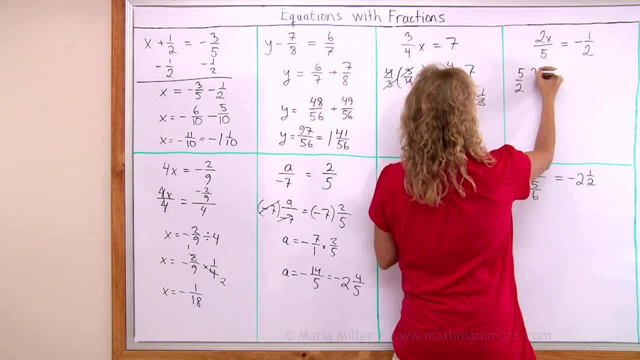 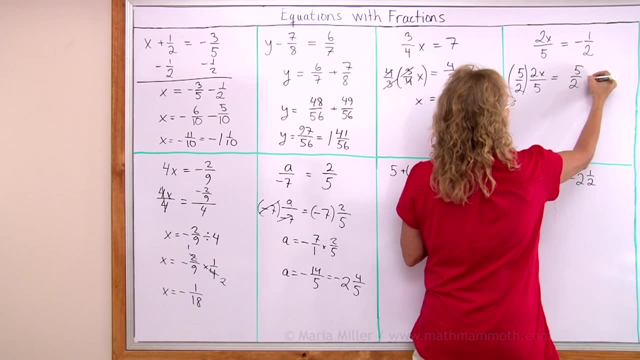 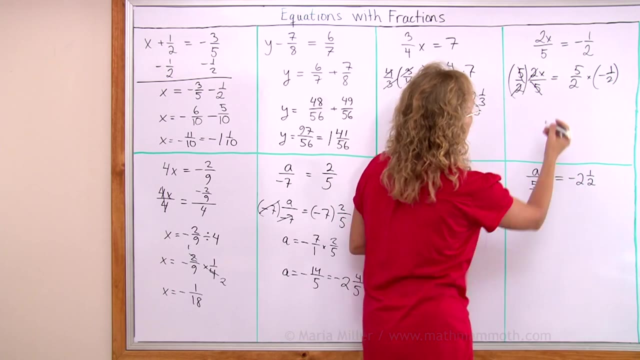 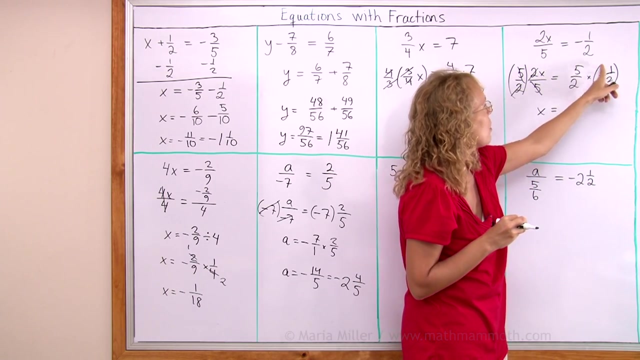 cancel. So we multiply it by 5 over 2, and then you have 2x over 5,. okay, And then here same thing. here 5 over 2 times negative 1 half. So now here everything cancels, except the x Over. here nothing simplifies. we just multiply 5 times 1. 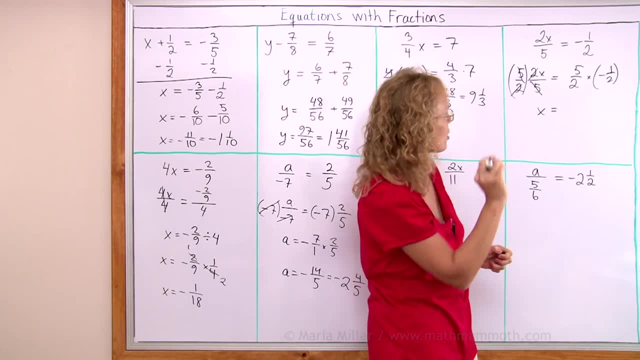 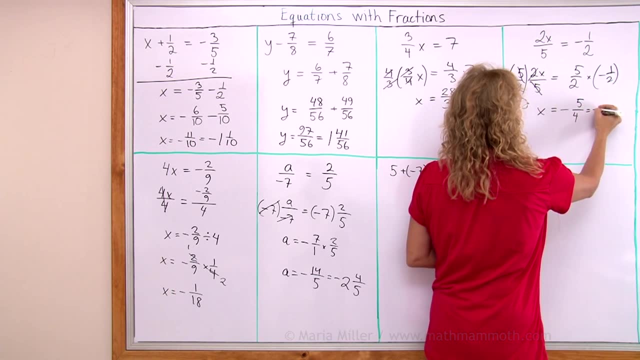 and 2 times 2.. The answer will be negative fraction, because this has positive times. negative, so I get negative. And then 5 over 4, which is negative. 1 and 1. fourth- This one here might look a little bit more complicated- 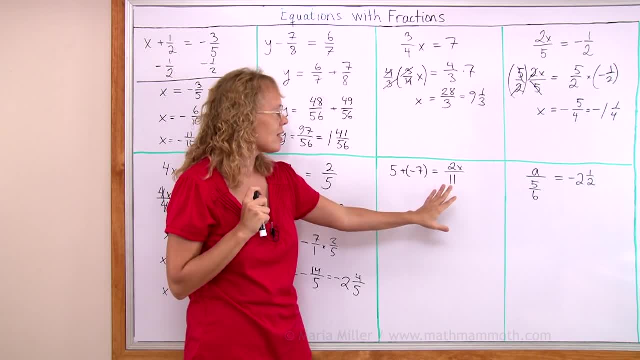 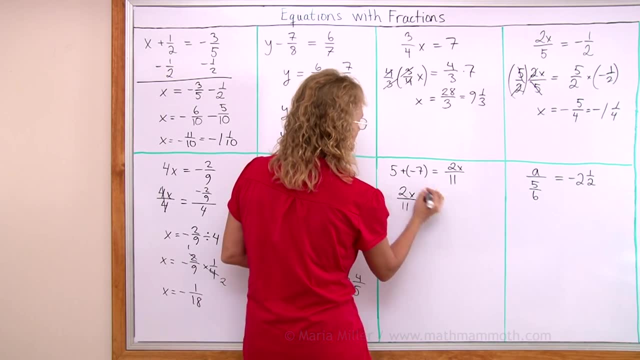 but it's not really. You see, I can flip this side so that I get my x and y. I can flip this side so that I get my x and y. I can flip this side so that I get my x on the left side. So I'll write it just: 2x over 11 equals this here on the other side. 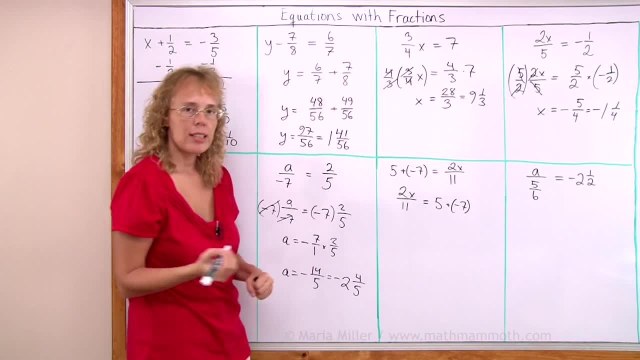 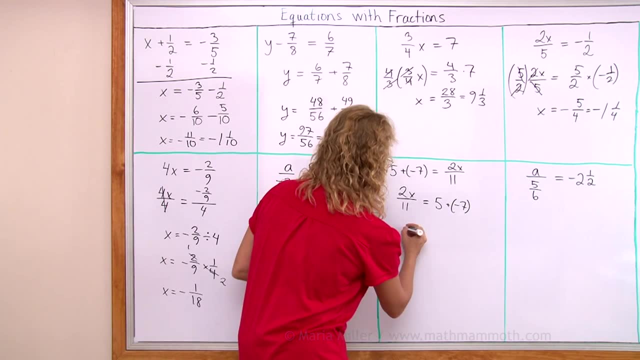 for starters, The next thing I can do is simplify. on the right side I can calculate 5 plus negative 7. That's negative 2, right. So I get 2x over 11 equals negative 2.. Now it is exactly like we had. 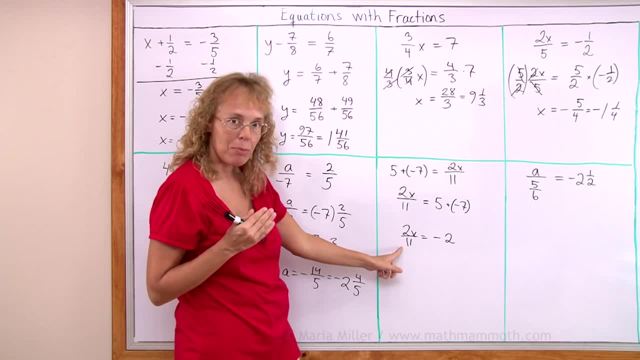 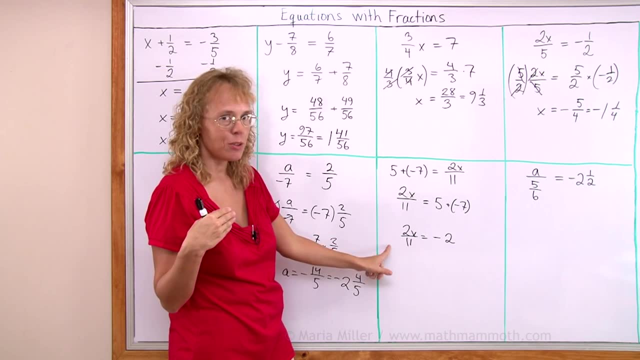 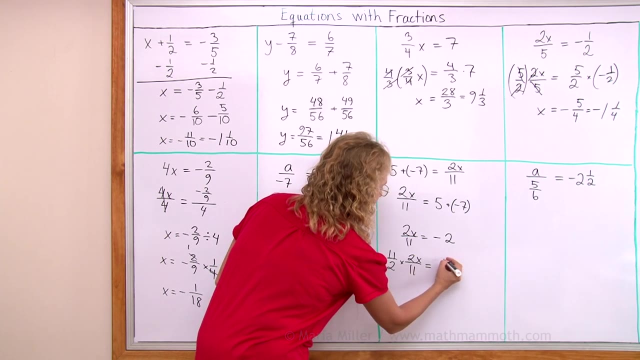 here and here We need to multiply so that these two elevenths here will cancel out. So we multiply by 11 over 2, right, 11 over 2 times 2x over 11.. On this side, 11 over 2 times negative: 2.. Those 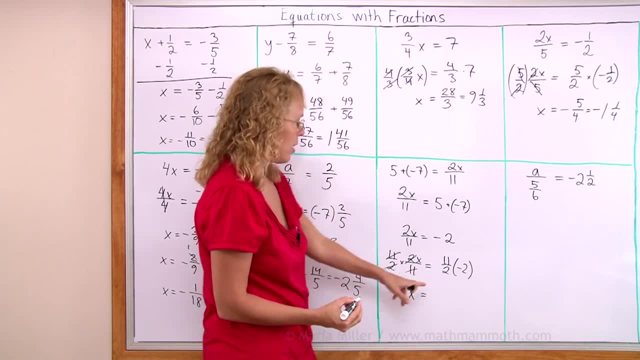 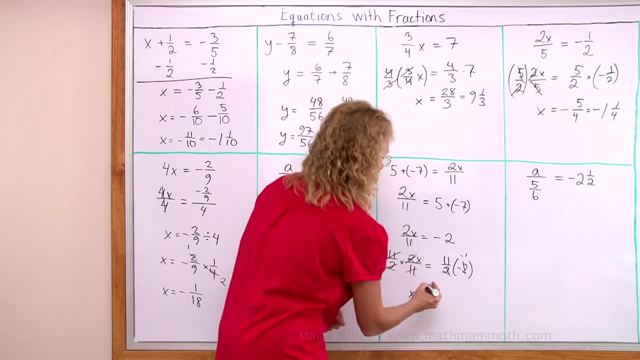 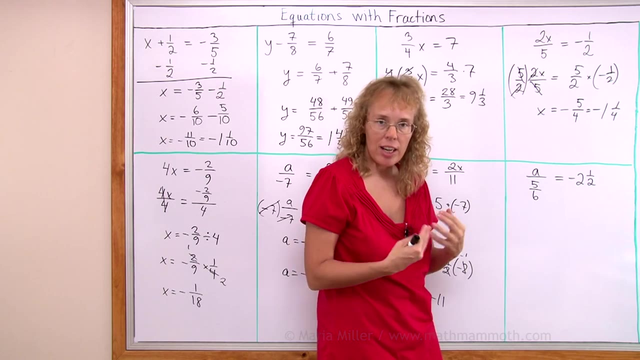 cancel. x is left alone Over here. 2 and 2 cancel 2.. So there's the negative 1, there now Negative 1. So we get negative 11.. A whole number, this time, Lastly a over 5 sixths or a divided by 5 sixths. Okay, so here's a variable divided by something. 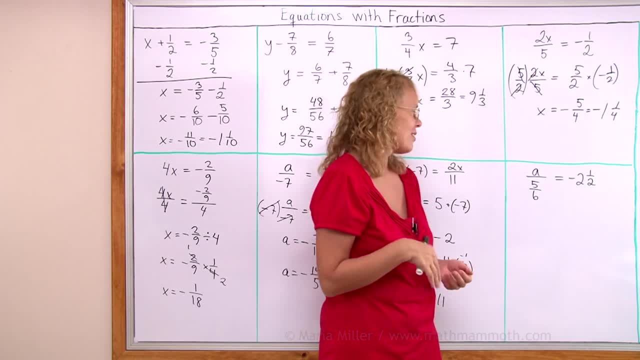 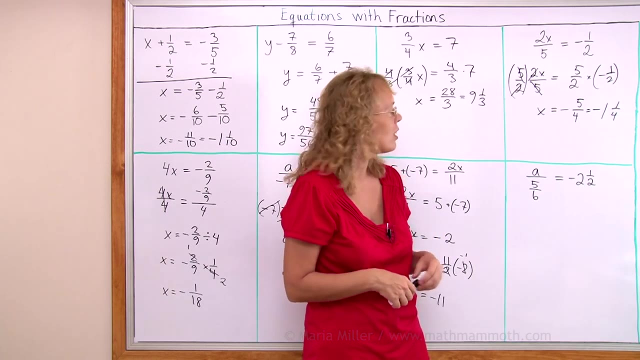 It's a division equation, so we would multiply, right. We would multiply by 5 sixths to solve the equation. Now, you don't normally see it written this way. Normally you would see 6a over 5.. Okay, but I chose it as an example of a complex fraction here. Multiply both sides by 5 sixths. 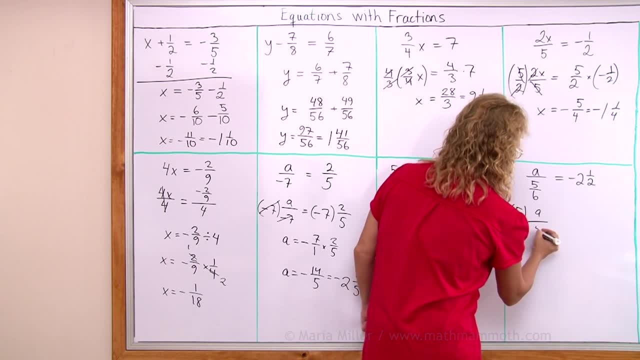 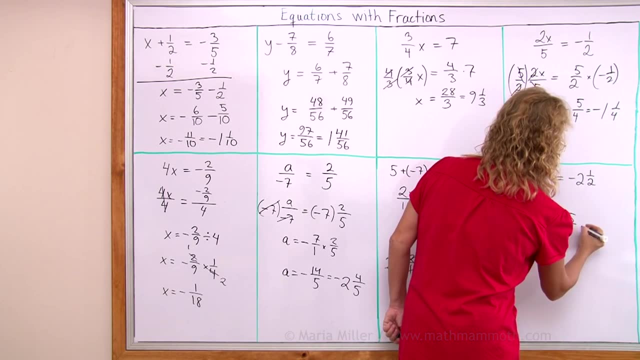 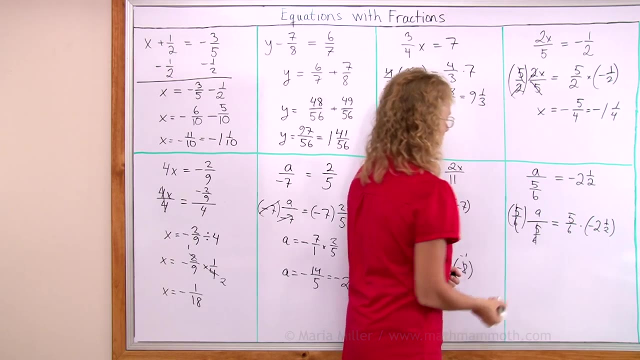 So 5 sixths times a over 5 sixths Looks kind of like that Equals. then over here on this side, 5 sixths times this negative 2 and a half. Okay, Over here these now cancel. a is left alone. Over here, a fraction.